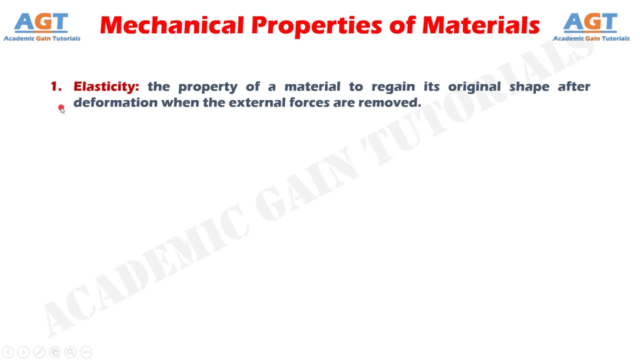 It is also called as the tensile property of the material. Proportional Limit: It is defined as the maximum stress under which a material will maintain a perfectly uniform rate of strain to stress, Though its value is difficult to measure. yet it can be used as the important applications for building precision instruments: springs. 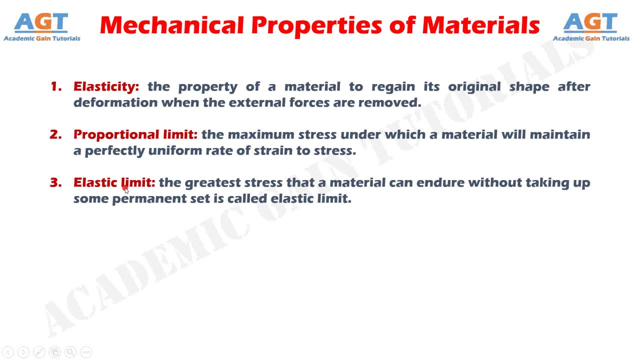 etc. Elastic Limit: Many metals can be put under stress slightly above the proportional limit without taking a permanent set. The greatest stress that a material can endure without taking up some permanent set is called elastic limit. Beyond this limit the metal does not regain its original form. 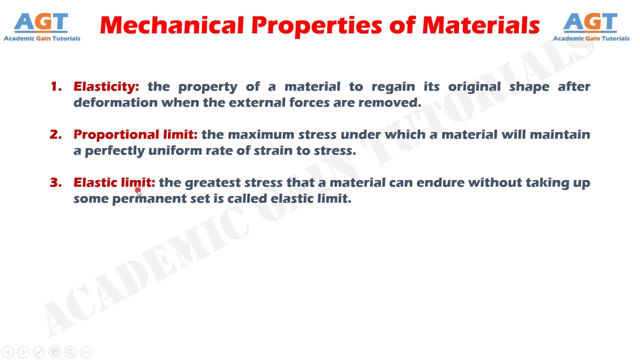 and permanent set will occurs. Yield point: Yield point is the load at which a solid material that is being stretched begins to flow or change shape, permanently divided by its original cross-sectional area or the amount of stress in a solid at the onset of permanent deformation. The yield point 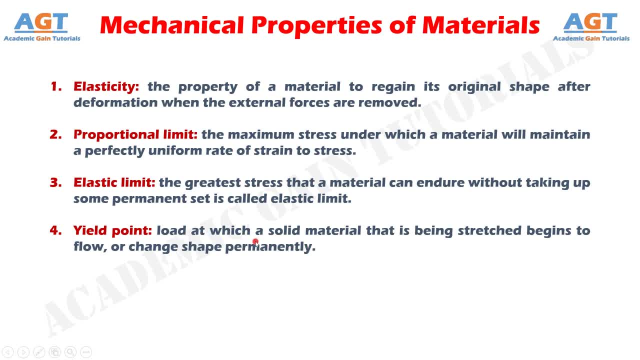 marks the end of elastic behavior and the beginning of plastic behavior. When stress is less than the yield point are removed, the material returns to its original shape. Strength: Strength is defined as the ability of a material to resist the externally applied forces with breakdown or 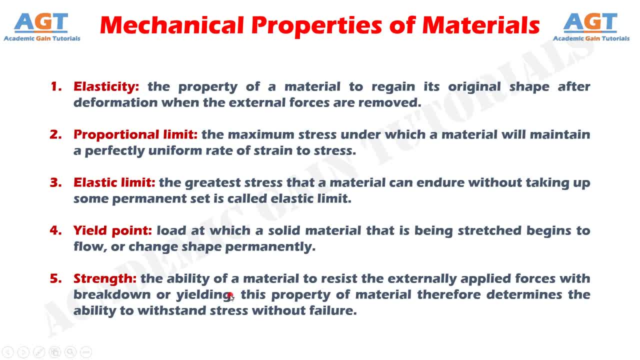 yielding The internal resistance offered by a material to an externally applied force is called stress. The capacity of bearing load by metal and to withstand destruction under the action of external loads is called stress- is known as strength. The stronger the material, the greater the load it can withstand. This 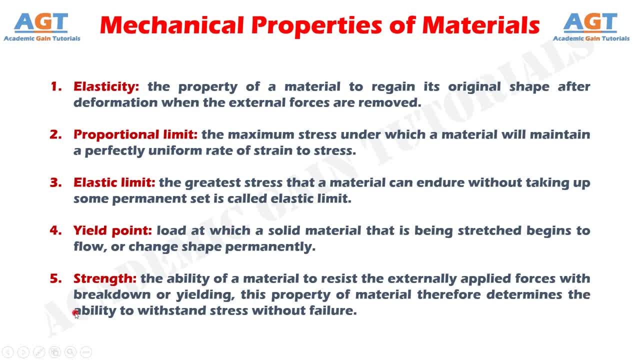 property of material therefore determines the ability to withstand stress without failure. Strength varies according to the type of loading. It is always possible to assess tensile, compressive, shearing and torsional strengths, The maximum stress that any material can withstand before destruction is called its ultimate strength. The tenacity of the material is: 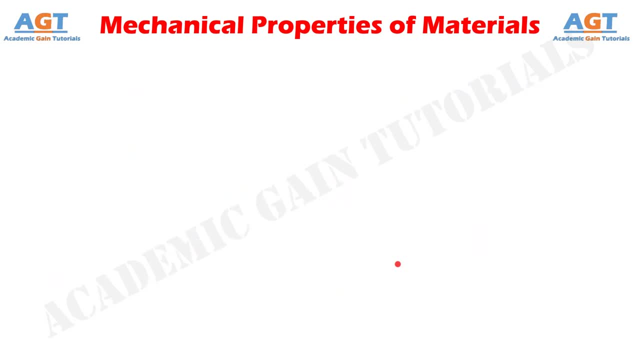 its ultimate strength in tension Stiffness. It is defined as the ability of a material to resist deformation under stress. The resistance of a material to elastic deformation or deflection is called stiffness or rigidity, A material that suffers slight or very less deformation. 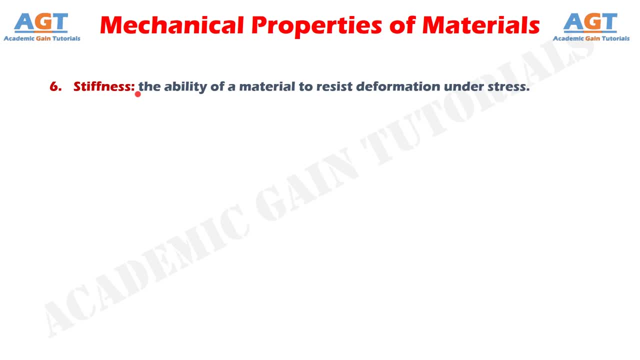 under load has a high degree of stiffness or rigidity. For instance, suspended beams of steel and aluminium may both be strong enough to carry the required load, but the aluminium beam will sag or deflect further. That means the steel beam is stiffer or more rigid than aluminium beam If the material behaves. 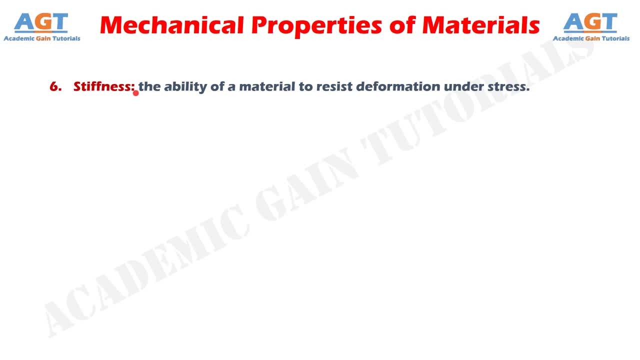 elastically with linear stress strain relationship. under Hooke's law its stiffness is measured by the Young's modulus of elasticity. The higher is the value of the Young's modulus, the stiffer is the material In tensile and compressive stress. it is called modulus of stiffness or modulus of. 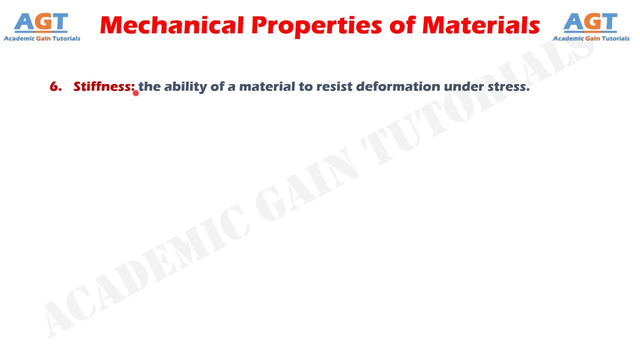 elasticity In shear, the modulus of rigidity, and this is usually 40 percent of the value of modulus for commonly used materials. In volumetric distortion, the bulk modulus Plasticity. Plasticity is defined the mechanical property of a material which retains the deformation. 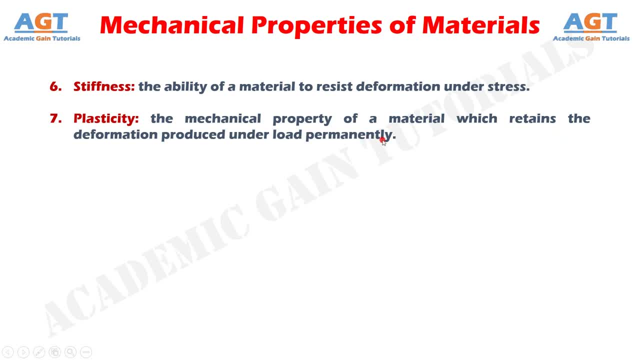 produced under load permanently. This property of the material is required in forging, in stamping images on coins and in ornamental work. It is the ability or tendency of material to undergo some degree of permanent deformation without its rupture or its failure. Plastic deformation takes a certain amount of time to deform. It is the ability or tendency of material to undergo some degree of permanent deformation without its rupture or its failure. Plastic deformation. 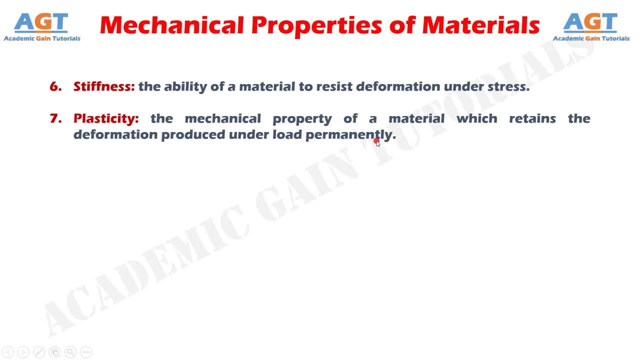 takes a certain amount of time to deform. It is the ability or tendency of material to undergo some degree of permanent deformation without its rupture or failurexus place only after the elastic range of material has been exceeded. such property of material is important in forming, shaping, extruding and many other. 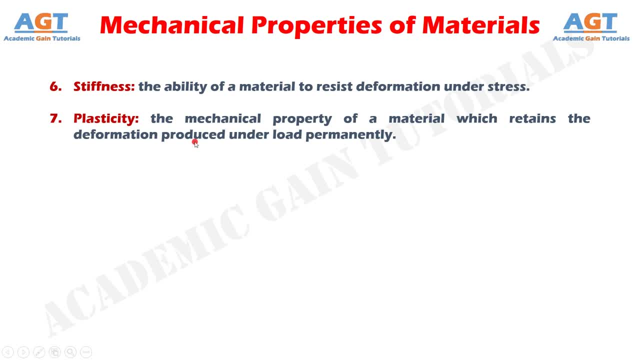 hot or cold working processes. materials such as clay, lead, etc. are plastic at room temperature and steel is plastic at forging temperature. this property generally increases with increase in temperature of materials. ductility- ductility is termed as the property of a material enabling it to be drawn into wire with the application of tensile load. A ductile material must be strong in plastic. 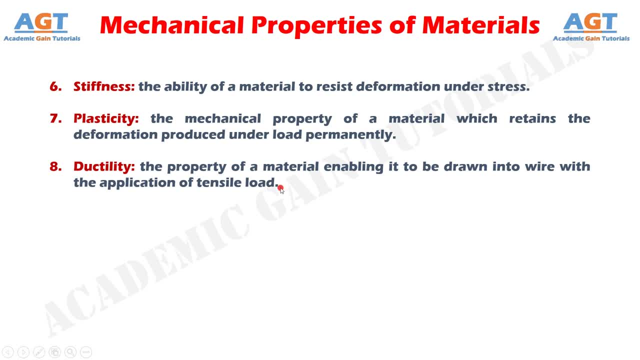 The ductility is usually measured by the terms percentage elongation and percent reduction in area, which is often used as empirical measures of ductility. The materials those possess more than 5% elongation are called as ductile materials, The ductile material commonly used in engineering. 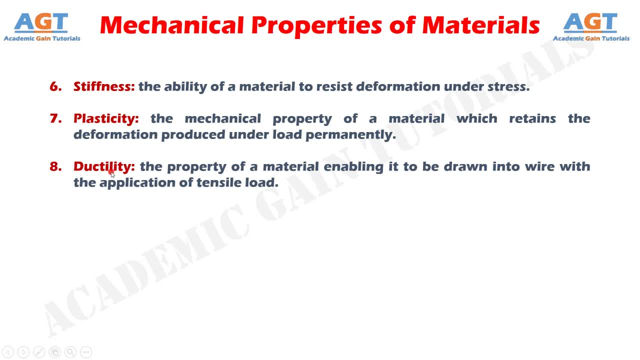 practice in order of diminishing ductility are mild steel, copper, aluminum, nickel, zinc, tin and lead Malleability. Malleability is the ability of the material to be flattened into thin sheets under applications of heavy compressive forces without cracking by hot or cold working. 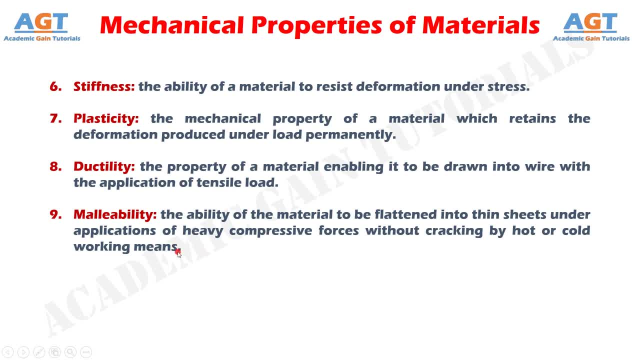 means. It is a special case of ductility which permits materials to be rolled or hammered into thin sheets. A malleable material should be plastic, but it is not essential to be so strong. The malleable materials commonly used in engineering practice in order of diminishing 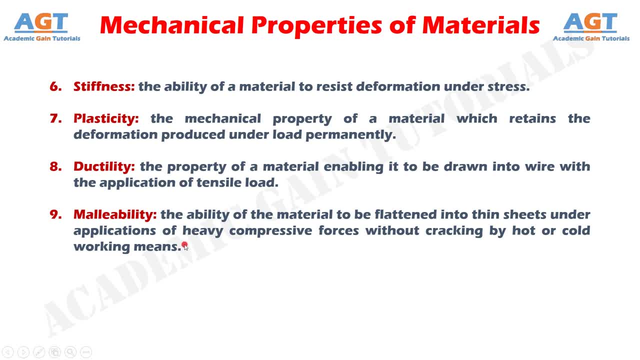 malleability are lead, soft steel, wrought iron, copper and aluminum. Aluminum, copper, tin, lead steel, etc. are recognized as highly malleable metals. Hardness: Hardness is defined as the ability of a metal to cut another metal. A harder metal can. 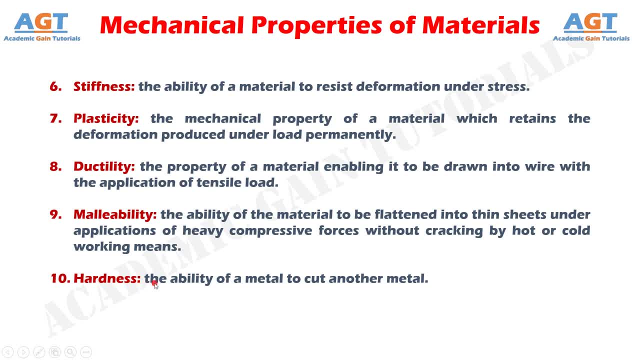 always cut or put impression to the softer metals by virtue of its hardness. It is a very hard metal to cut. It is a very hard metal to cut. It is a very hard metal to cut. It is a very important property of the metals and has a wide variety of meanings. It embraces many 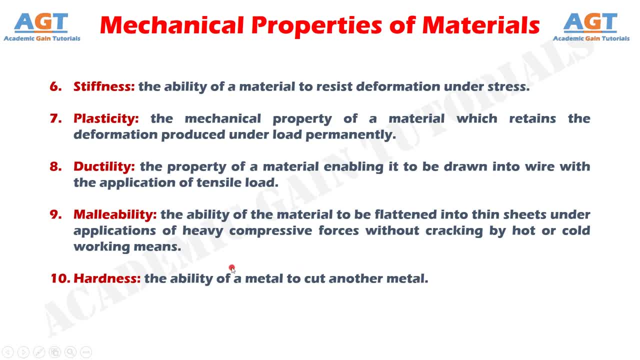 different properties, such as resistance to wear, scratching, deformation and machinability, etc. Brittleness. Brittleness is the property of a material opposite to ductility. It is the property of breaking of material with little permanent distortion. The materials having less than 5%. 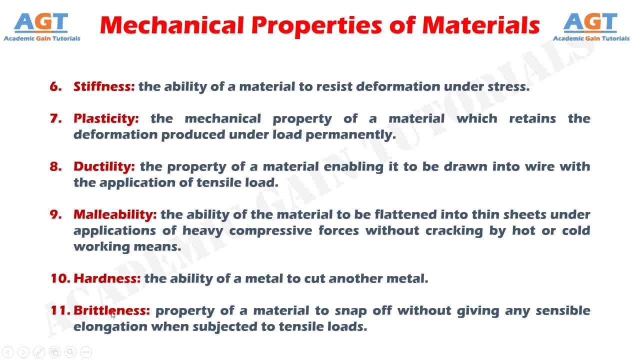 elongation under loading behavior are said to be brittle materials. Brittle materials, when subjected to tensile loads, snap off without giving any sensible elongation. Glass, cast iron, brass and ceramics are considered as brittle material. Thus brittleness is the property of a. 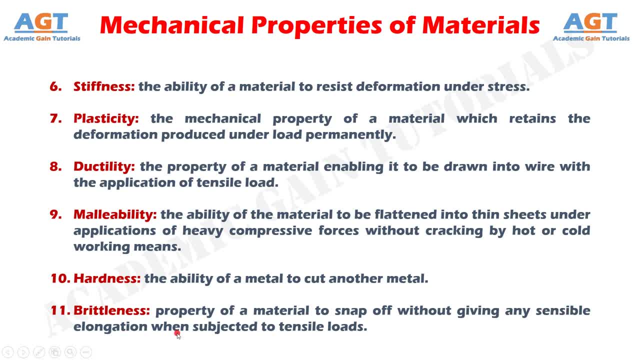 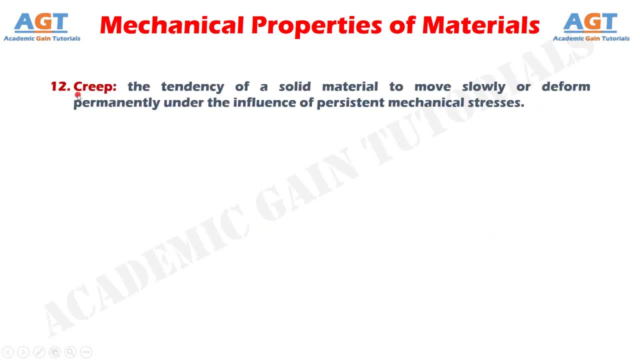 material to snap off without giving any sensible elongation when subjected to tensile loads Creep. When a metal part when is subjected to a high, constant stress at high temperature for a longer period of time, it will undergo a slow and permanent deformation in form of a metal part. 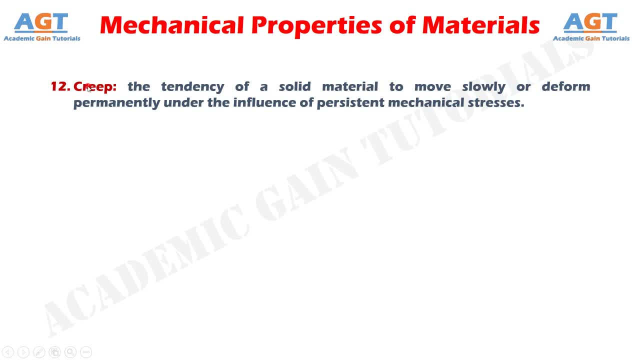 Creep is the property of a crack which may further propagate further towards creep failure called creep, In other words creep, sometimes called as cold flow- is the tendency of a solid material to move slowly or deform permanently under the influence of persistent mechanical 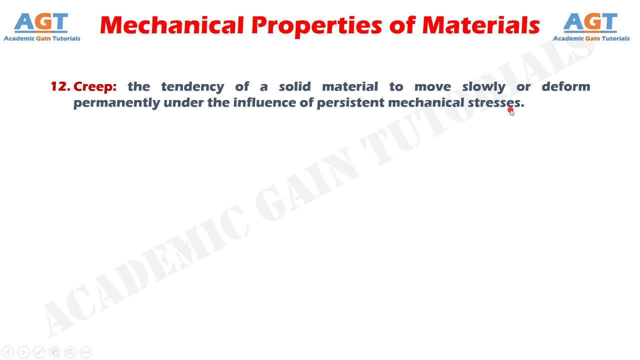 stresses. It can occur as a result of long-term exposure to high levels of stress that are still below the yield strength of the material. Formability: Formability is the ability of a metal workpiece to undergo plastic deformation without the help of a metal part. This is the